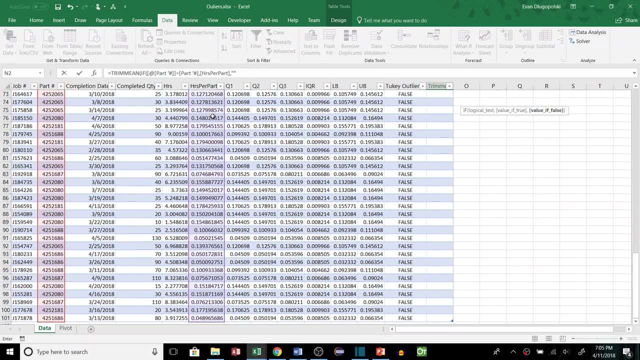 this array of values, And then the false will just enter a blank value because it should always be true, And then the percent we'll use is 10%. so 0.1.. And 10% is a pretty typical value, but you. 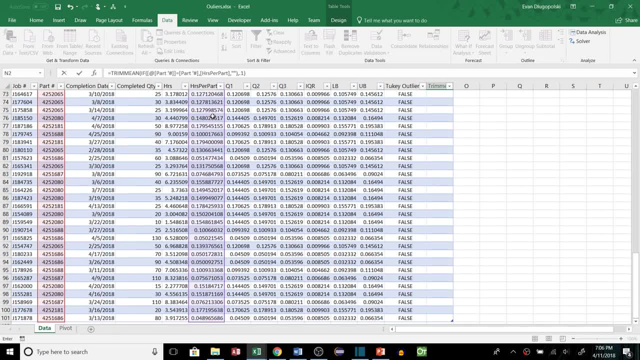 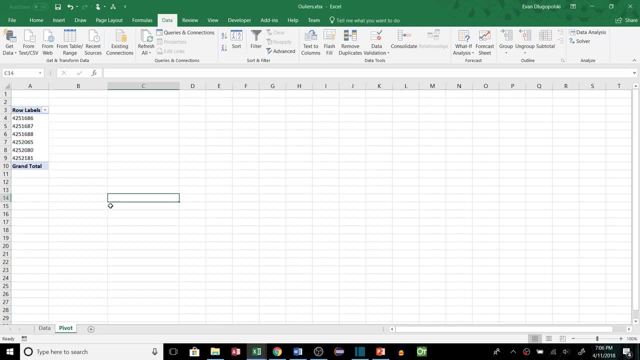 might also want to use 20% or something like that. That might be a bit extreme, depending on your sample size, But we'll hit control, shift, enter to make that an array function. You'll notice these little brackets, So let's take a look at the pivot table. This will refresh our data, so everything is. 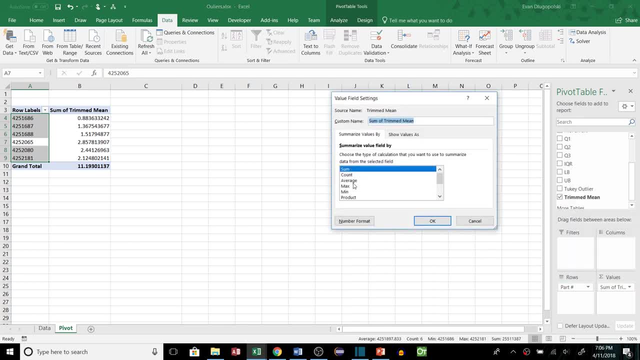 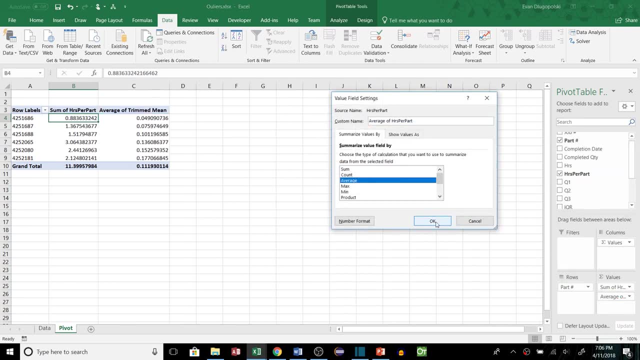 up to date And then we'll drop in the trim mean value and make that an average. And just for comparison, let's look at the hours per part. So we'll take a look at the hours per part and we'll take the average of that. So this will be the original mean And we can see that they're pretty. 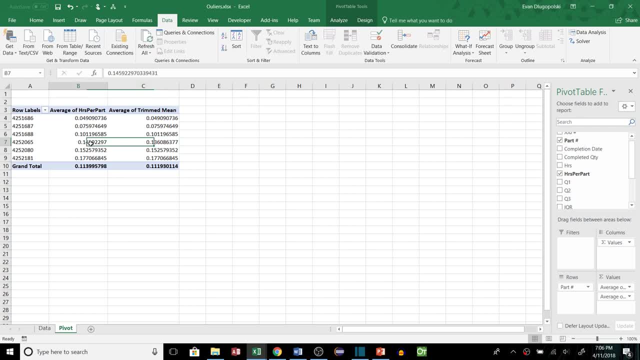 much the same, except for this one value. So that was the only case where it took out some values in order to give us a trim mean. The reason it only affected this part number is because we use the value of 10% for our trim percentage. That means it takes off 5% of the count. 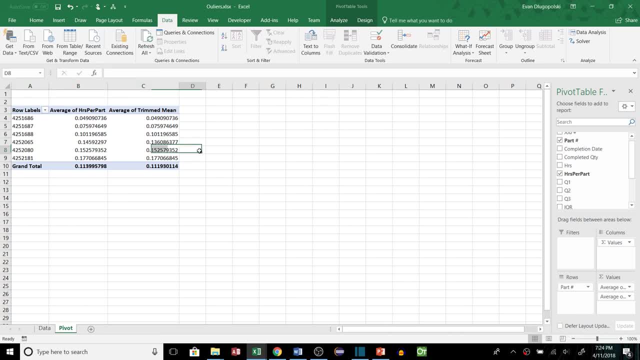 or 5% of the samples from both ends of the distribution. So this part number is 10% and we'll take the average of that. So this will be the original mean And we can see that they're pretty much the same except for this one value. So that was the only. 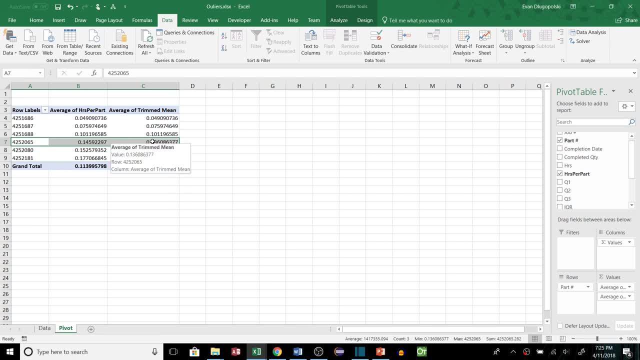 case where it took out some values in order to give us a trim mean. This part number was the only one that had more than 20 samples, So 5% of 20 is 1.. So that means it takes off one value from each. 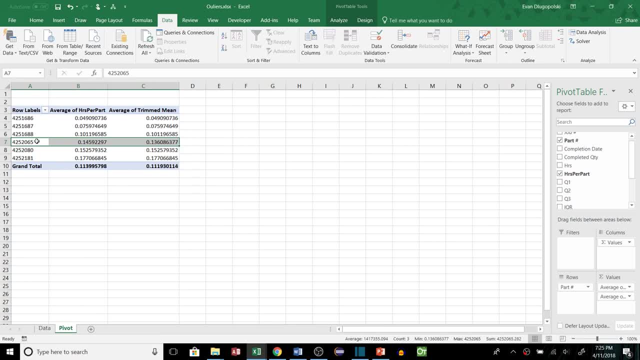 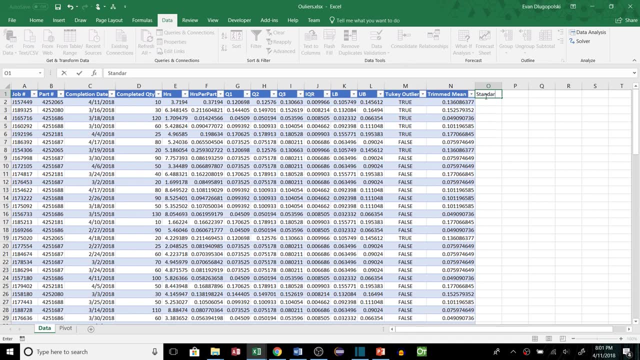 end If it's less than 20, it actually rounds down, so it won't actually trim any values. All right, next let's look at the standard z-score method for detecting outliers. So, standard z-score, we'll add a column, And for this we're actually going to add another column. 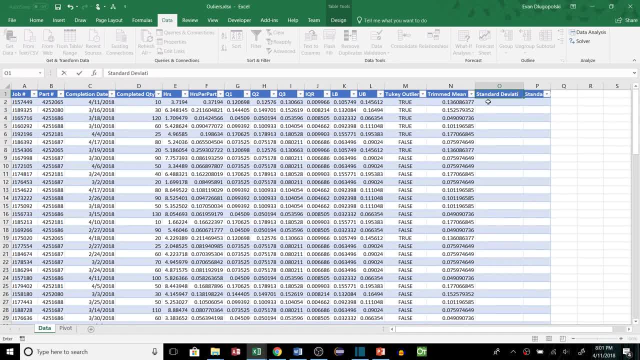 and this is going to be the standard deviation, And the standard deviation is is used to calculate a z-value, So we'll need to calculate that first And again we're going to use an array method, We're going to say standard deviation and we'll want. 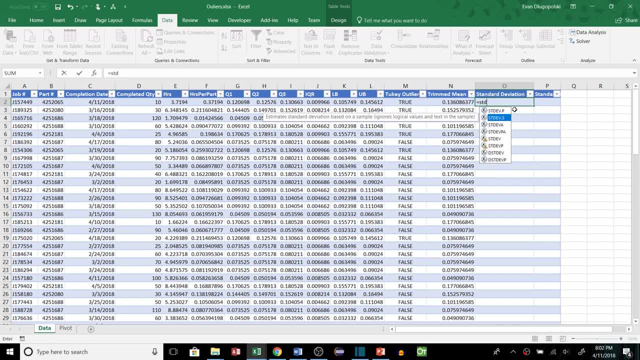 there's two here. This is for the population standard deviation. This is for the sample standard deviation. We're going to use the sample And then we'll do the standard deviation. If same thing, we're going to match our part number to the array, The value of true is going to be. 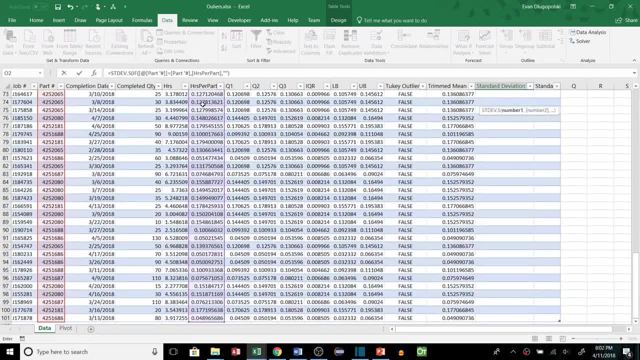 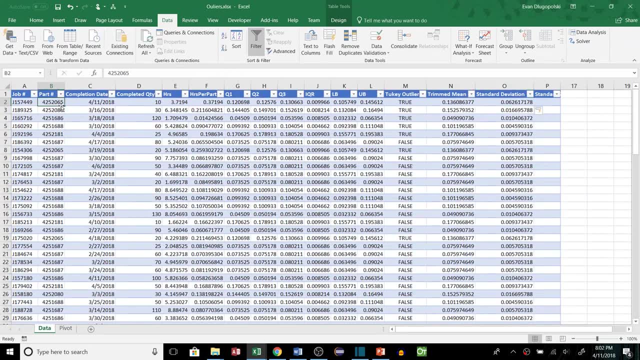 our part values. blank for false control shift: enter oops, this in the parenthesis. Okay, there we go. This is going to be the standard deviation for each part number. We'll also need to add in the mean, so the original mean or average. This is going to be. 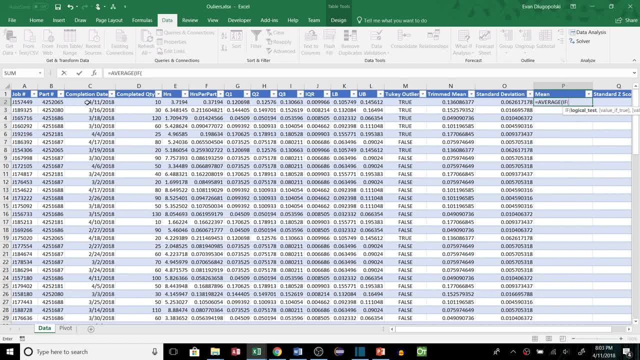 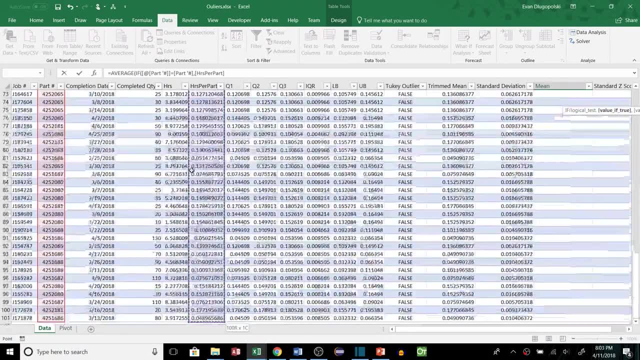 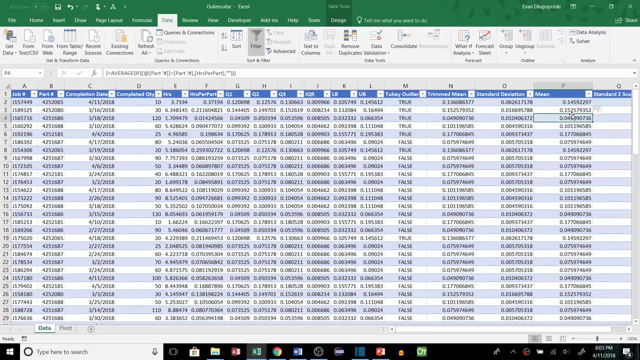 average and if this part number equals the array, then use the hours per part array. value of false is blank. Close off the average and hit control shift- enter. So now that we have a standard deviation and mean, we can calculate the standard z score. 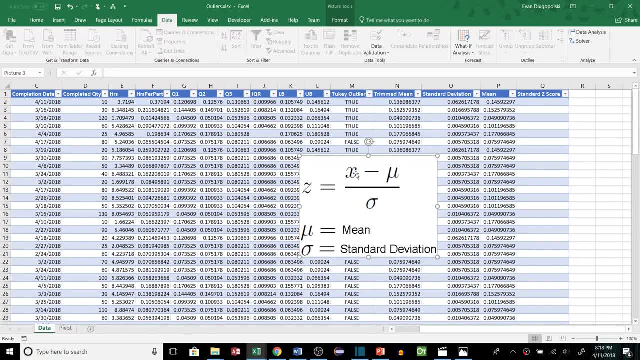 And z score is calculated with this equation. Basically, we're finding out how many standard deviations are there between a given sample and the mean of that sample. So we could just enter in or set up an equation manually. but Excel also has a build-in function for calculating this. 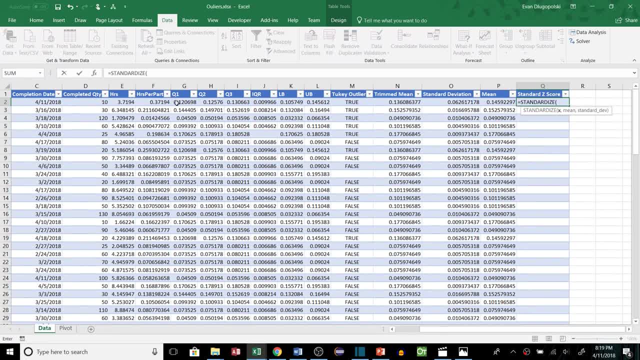 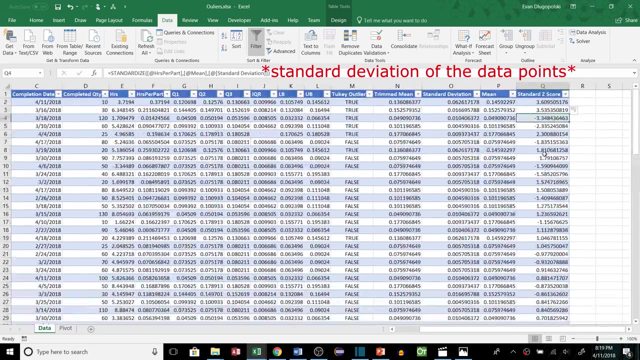 So we can say: equals mean standardize, find the X value for that sample, compare that to the mean of all the samples and then feed the function the standard deviation for these samples and then when we hit enter, there we get our z-score values. so if you remember, 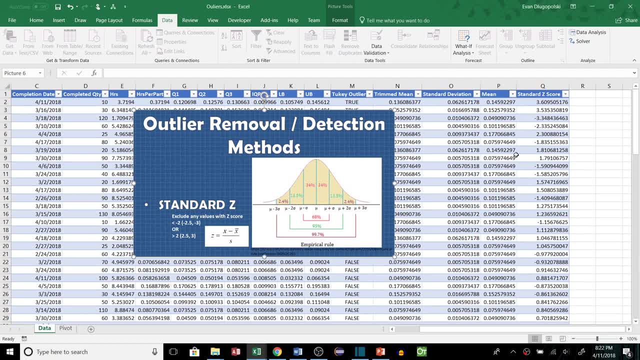 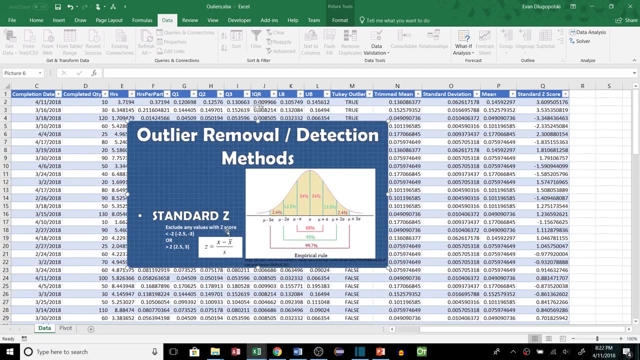 from the last video. then I said that we can determine outliers by using the z-score and setting a limit for the number of standard deviations that were allowing data to be considered non outliers. so I said we could use plus or minus two, two and a half or three standard deviations or z-score values. so 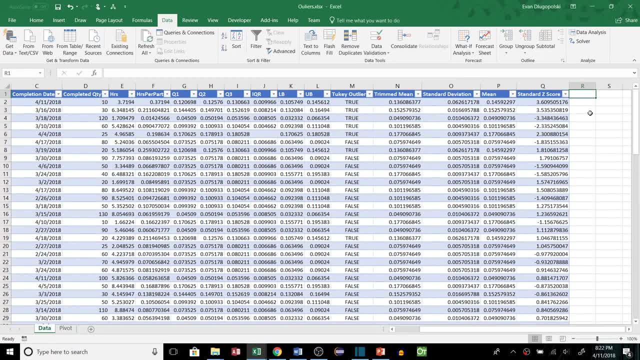 let's just use three as our limit on the z-score value. so let's say z-score outlier for that. then we'll just set up an if statement. say: if the absolute value of this is greater than three, true, and if not, then false. so now we can go back to our pivot table and see how. 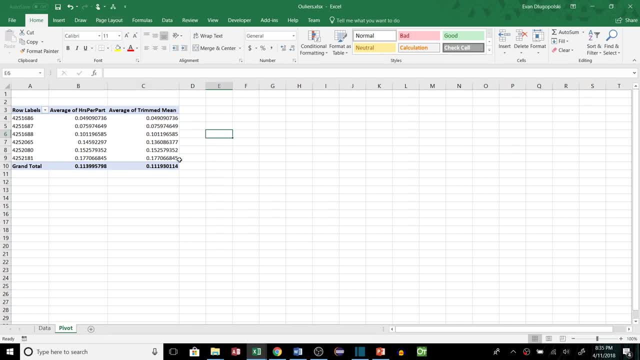 the mean changes, whether or not we include z outliers. so let's just kind of copy and paste these down so we can compare things. so this is the original mean, original mean, and then we'll say trim mean. and now, if we add a slicer to our pivot table to look at Z outlier values, we only want to 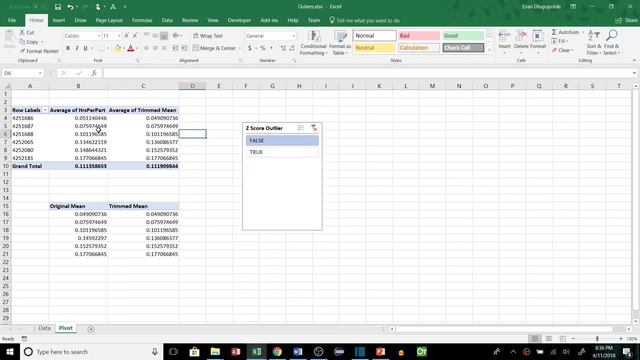 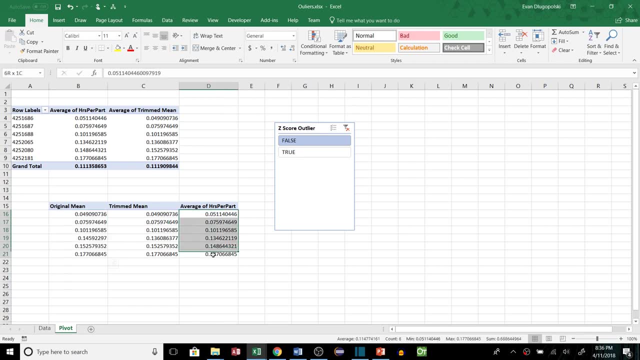 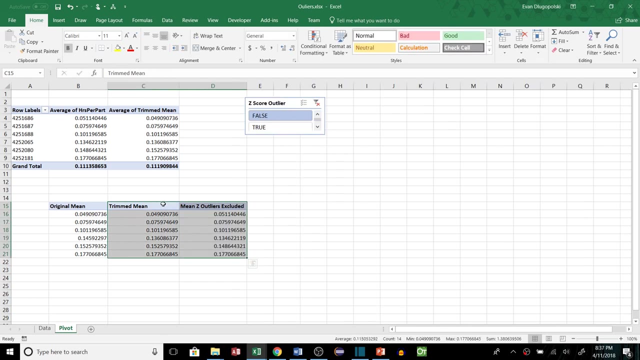 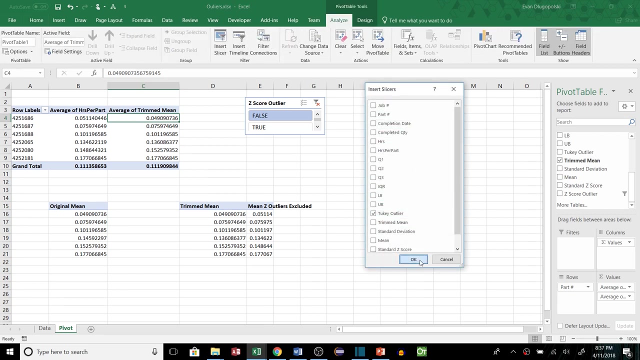 look at values that are false. So if we basically exclude any Z outliers, we can compare those values to our original mean. So there's our original mean. here is our mean with the Z outliers excluded. Then let's actually add in the Tukey outliers so we can compare that as well. So for Tukey outliers, add that in. 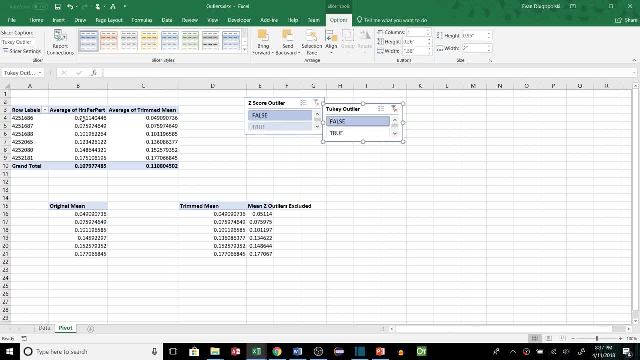 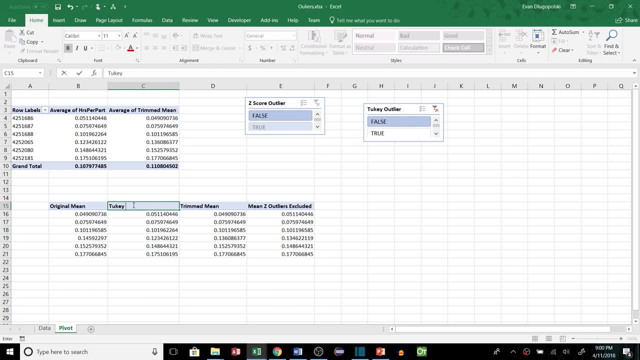 there, and we want those to be false and that to be true. So let's look at what that looks like. So now we can start to see how each method returns different results. So now let's look at the last method, which is going to be the modified. 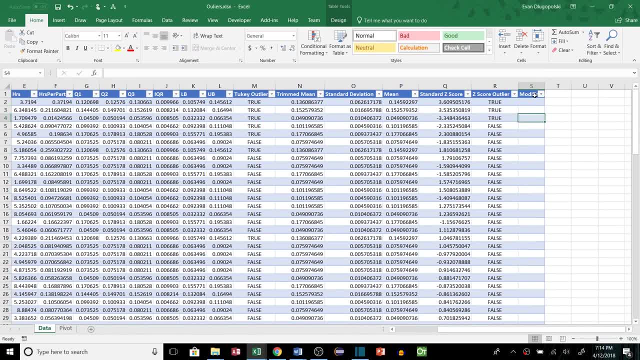 z-score. This one is tricky, but it's pretty robust, so this is one of my favorites. It works pretty well for small sample sizes, and it ends up returning similar results to the Tukey method as well, because it uses median values to determine all of them. 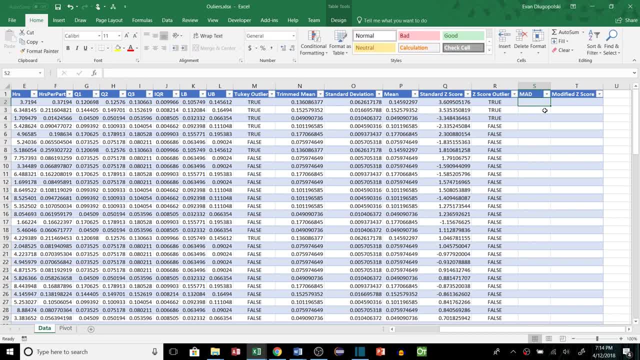 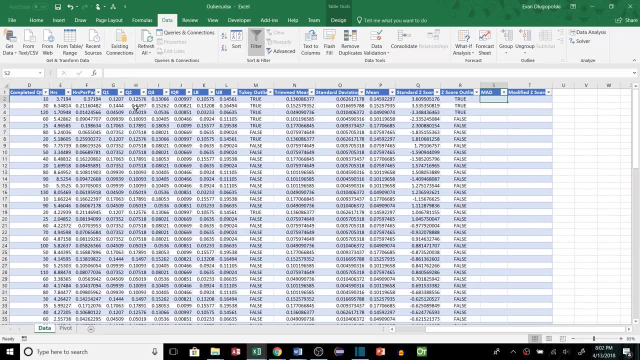 So we're going to need to add two columns here. We're going to say the MAD and modified z-score. So the MAD is going to be the median absolute deviation of each data point from the median. So that's kind of hard to explain. so I'm 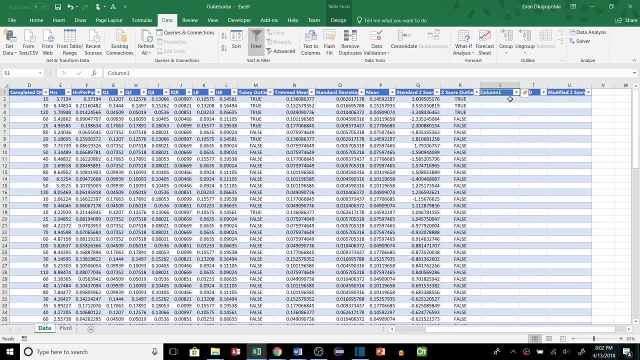 actually going to add another column which will hopefully make it a little bit easier to understand. So this is going to be the median, or actually the absolute median deviation. So now this value is going to be the difference from our data point and the absolute deviation. 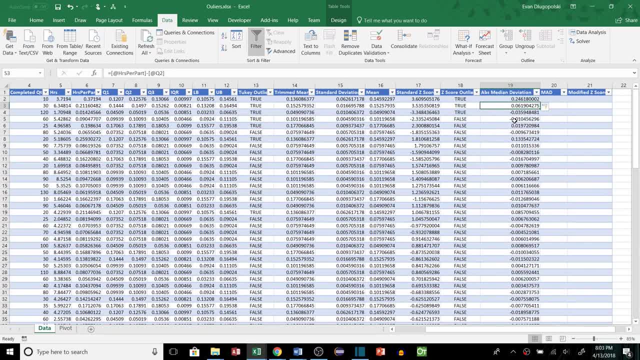 So we'll add that. Actually, sorry, that's the absolute value of that. So we're not concerned with direction, we're just concerned with how far our data point is from the sample median, And the MAD then is going to be another array function. 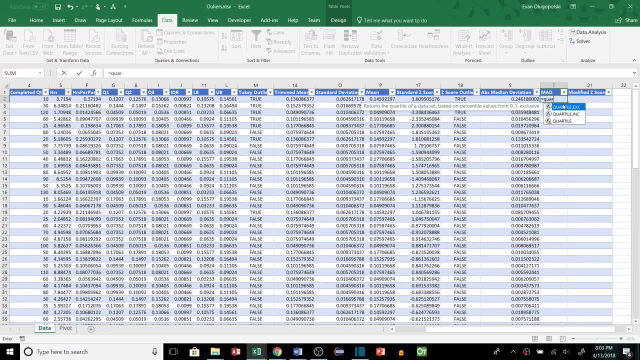 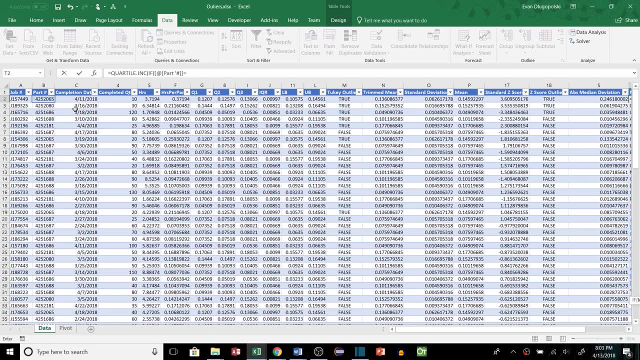 We're going to take the median of these values. We'll go quartile, just because I like to use that formula, And then this would be another array function. So we'll say if this part number matches the part array again, then we're going to look at this. 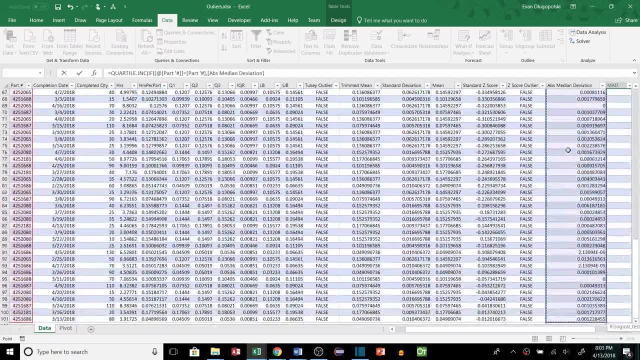 We're going to say, if群 is equal to or equal to 0,, if it contains an absolute deviation value- 0, then we're going to look to our absolute deviation values. If not nothing, Close off the if statement and then tell the quartile. 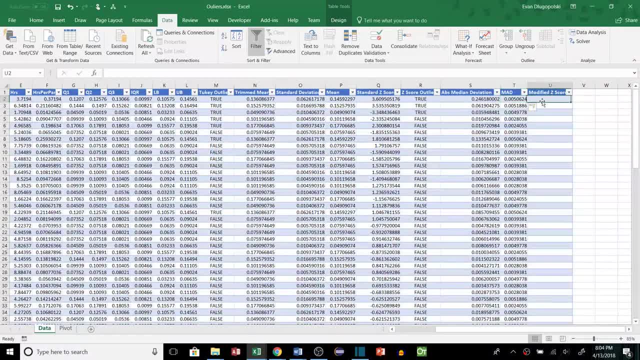 function which quartile we're looking, And that's the second quartile for the median. Then hit explore, short enter for that And this is our median absolute deviation. So this tells us how far each data point is from the median. So in order to calculate the modified Z-score now, if we look back at our formula from頻, our last video here, the modified Z-score equals our absolute deviation of our action. but if any data point is double and if your MAD is 20%, video will 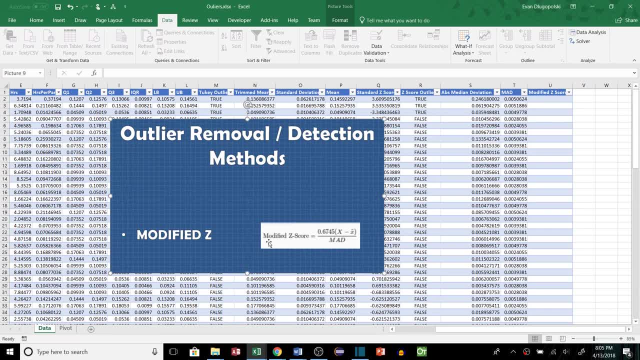 be connected to the consolidated Media and in turn, saved. it is a control. this constant times the difference between the data sample and the sample median divided by the MAD. Let's build this formula into our table here. We'll say 0.6745 times the difference of our data sample and our 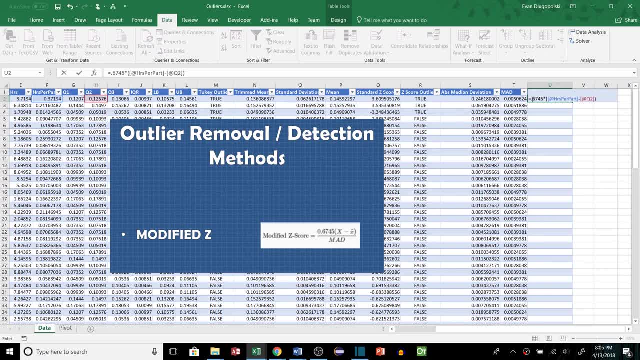 median quartile 2, and then all of that divided by the MAD, And then if we hit enter there, these are going to be the values for a modified z-score. The last thing we need to do is add the column to say if it is a mod z-score outlier. So 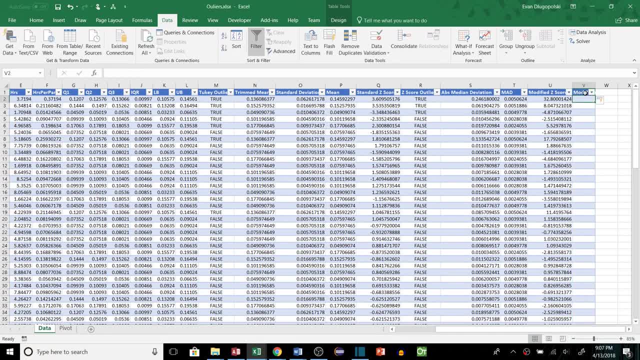 we'll add a column here, say mod z-outlier. We'll write a quick if statement to say if the absolute value of this is greater than 3.5 is typically the value used as a threshold for outliers when using the modified z-score method. So if it is, 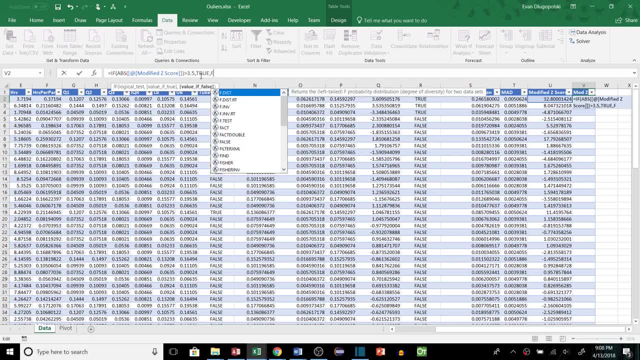 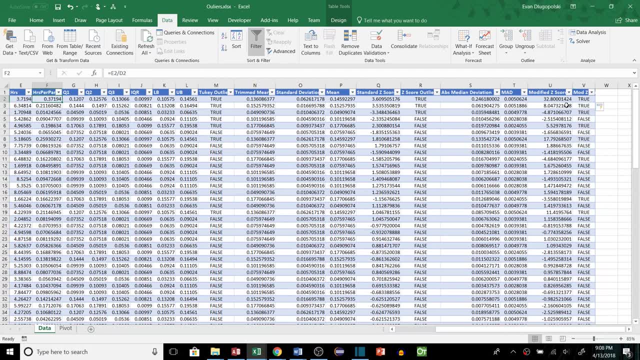 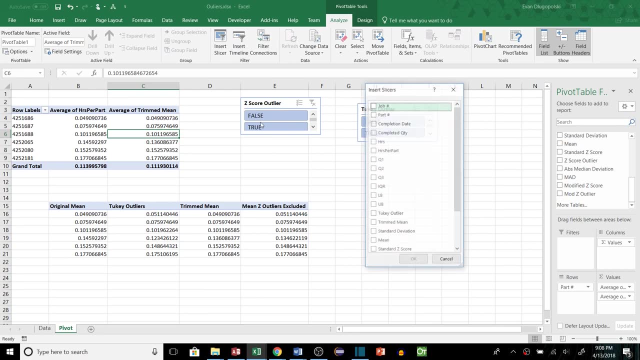 greater than 3.5, then we're going to return true to say yes it is an outlier, and if not, false, it is not an outlier. and then now we have identified our mod z outliers so we can go to our pivot table quick and take this filter off, refresh our data here. we want to add a slicer here so we can filter. 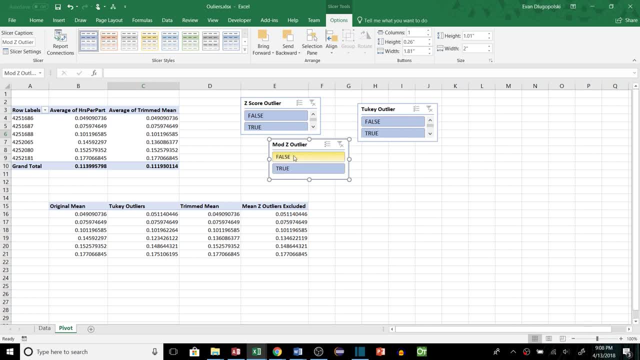 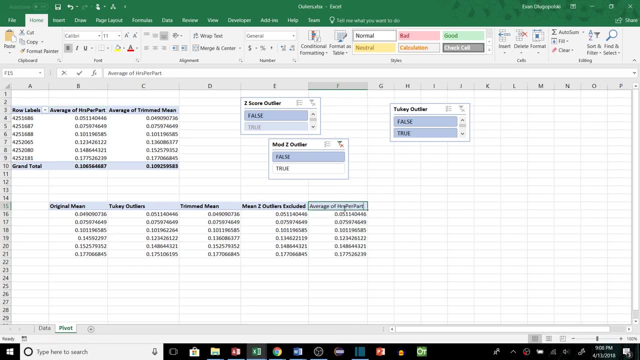 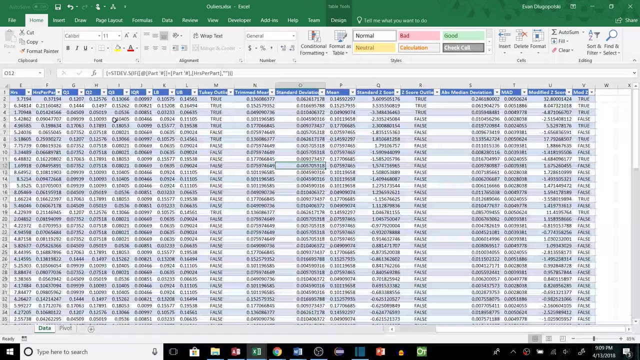 out the false values or the true values to filter out the outliers. so we'll just select just the false. here is the mean after modified z outliers have been removed. so there are our results. so i'm sure some of you might have been wondering why we were using array functions. they can be a little. 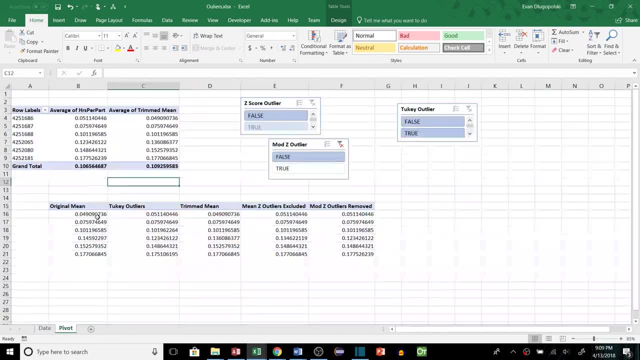 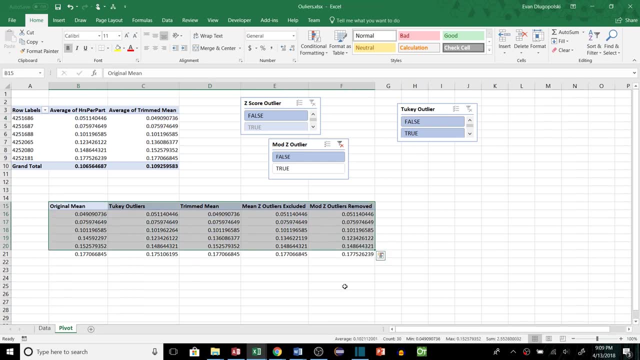 bit tricky. but the reason we need to use them is because we're trying to summarize our data by part number to get an average excluding these certain outliers. that was kind of the overall goal of this, just to kind of compare the different methods and see what they do for identifying. 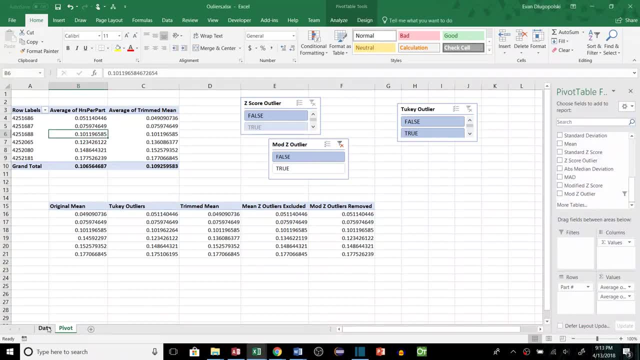 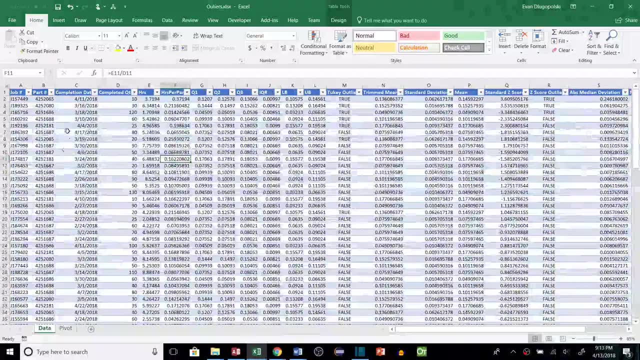 outliers, outliers how they change the mean things like that. Then one other note: just be cautious of using these array functions in large data sets. They're very nice because we can kind of aggregate data by a different you know a category here, like we did for the part numbers. But if this 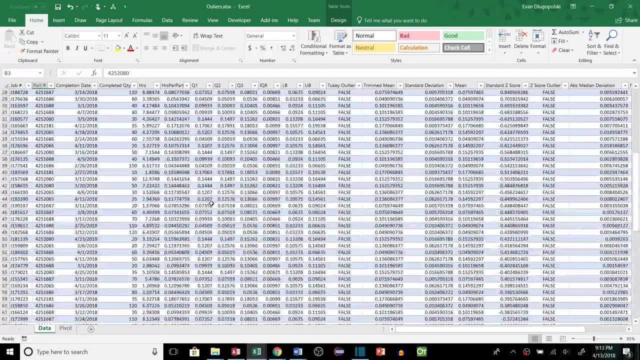 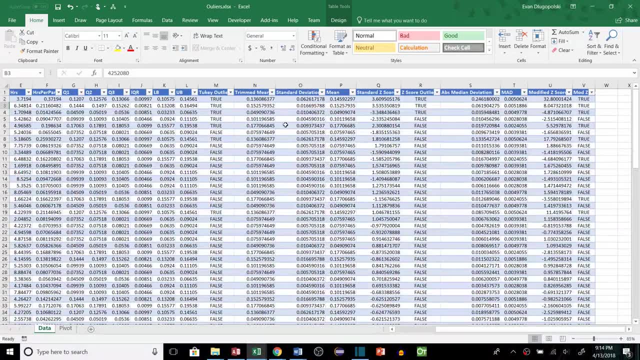 were a really long list of part numbers- definitely a lot bigger than this. I'm talking in like the thousands- It would really slow down the calculations that Excel has to do in order to calculate our values. So just be cautious of that. I've had spreadsheets before in the past. 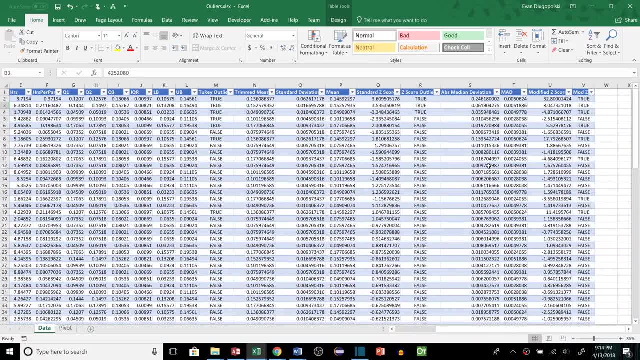 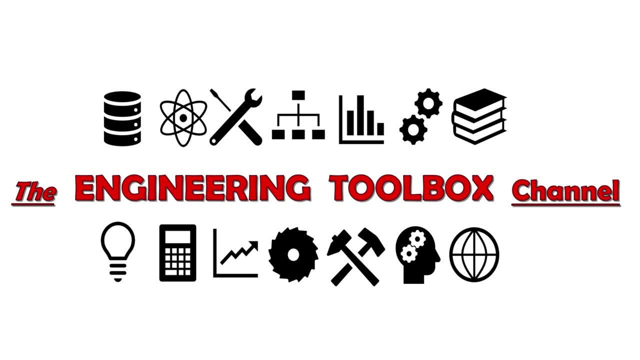 that are in the thousands of part numbers and it really gets bogged down. So just be cautious. All right, I hope you all enjoyed that one. To get more videos as they're released, make sure to hit that subscribe button. If you like this video, make sure to like and share.